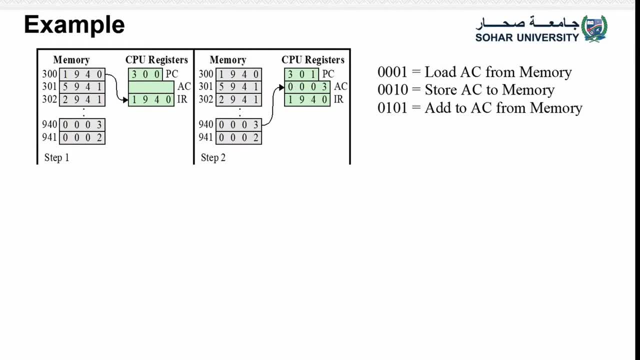 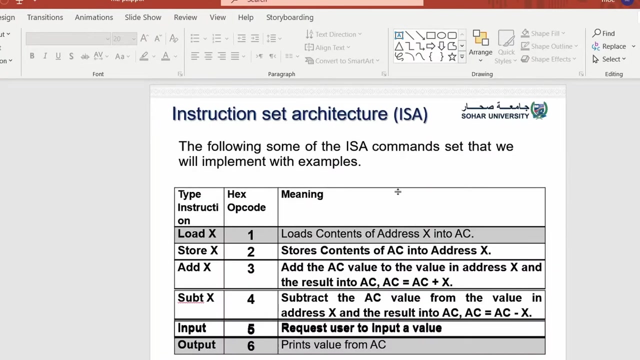 assalamu alaikum, in this video i'm going to be explaining how the cpu works and we are going to look at what are the instructions, what are the addresses and how the cpu handles them. so, first of all, you need to know that every instruction that the cpu does, either loading, 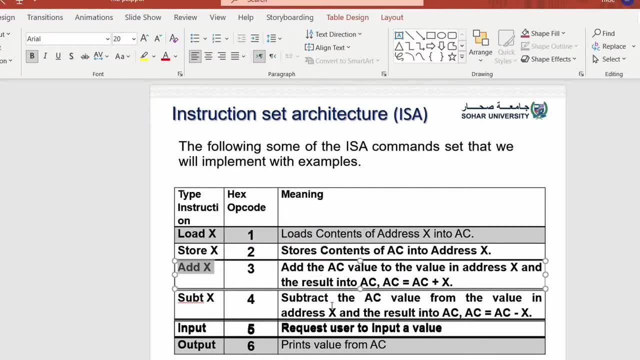 loading, storing, adding, subtracting, anything that these instructions are represented inside of the memory by a value, hexadecimal value. it's called an operation code, or opcode for short. okay, so load. x loads the contents of the address x, the address x, into the accumulator register. okay, so we have. 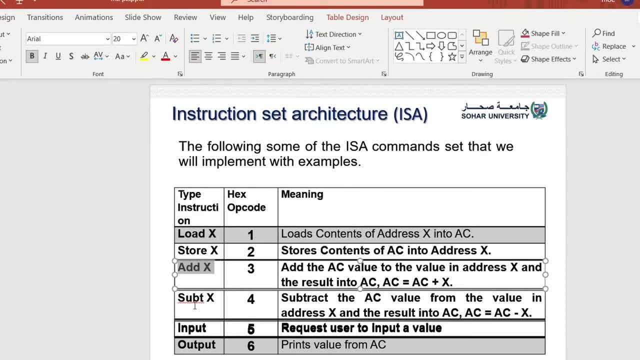 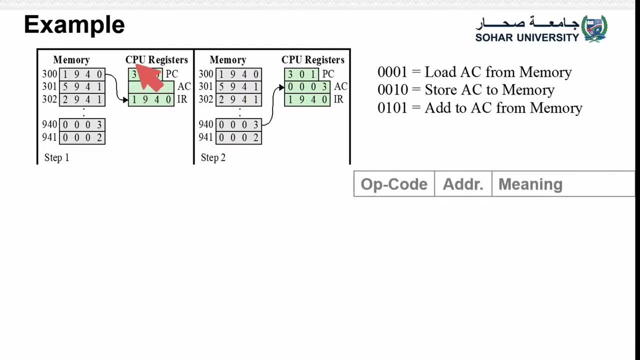 load, store, add instruction, subtract, and you can read about these. so what you want to know here is what each instruction does, and then you want to know what is the operation code for each instruction. okay, so when we go back here, you're gonna see here this number, these numbers, these are the addresses. 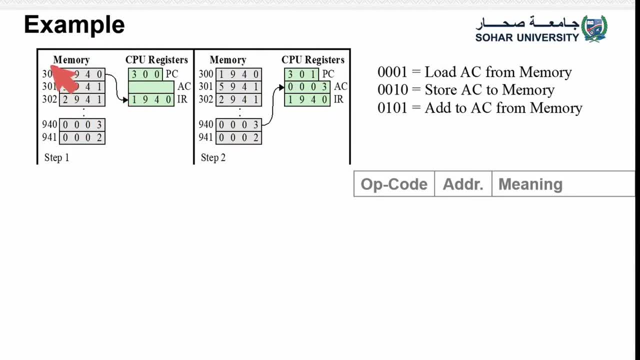 and now we address and one. so each, each container, these addresses are containers. okay, so the memory has containers. each container has an address. okay, kill the memory for her. can you talk to me? can you talk to me? you can feel, address, you know, and one come you had, did you make and fit them? and talk to me if you memory, okay, so 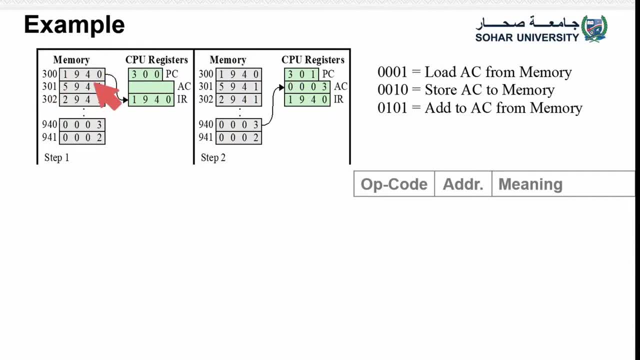 the 印 units hand is the operation code package, um. then when we go inside of the, when we go inside of the um address, we will see four numbers, four numbers, as you can see here. the first number here, these three first numbers for each address. it represents the um, the operation code. as you can see here, the 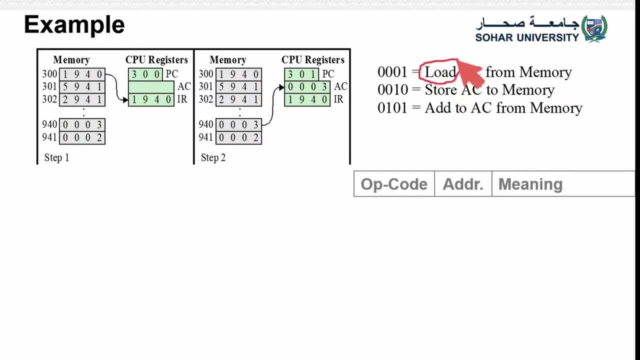 load instruction. the operation code load is one. okay, as you can see, it's here one. the the store instruction: okay, this is binary. okay, so if we convert this to by to to x, hexadecimal, it's going to be two. this is two and this is five. okay, and as you can see here, 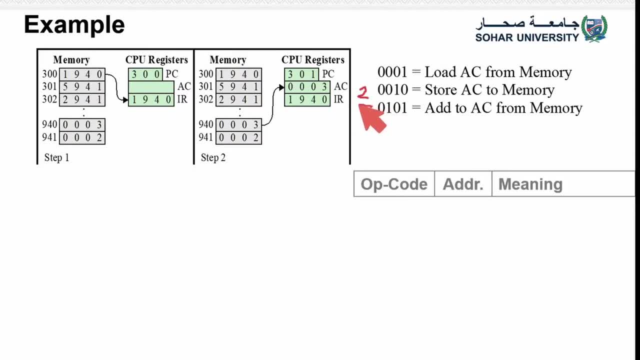 as you can see here, okay, as you can see here, this is a store, uh, add instruction and this is, as you can see here, store instruction inside of the accumulator register. okay, okay. so if we convert this to by, to x hexadecimal, it's going to be two. this is two and this is five. 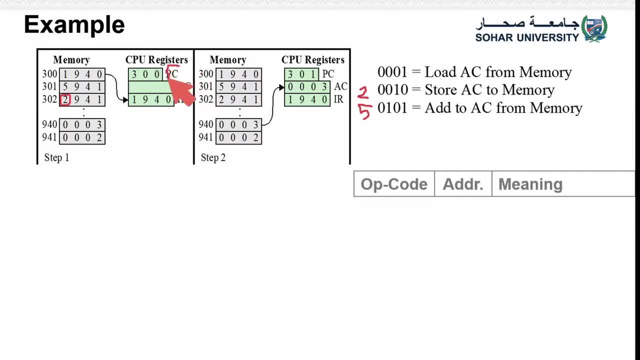 okay. so if we convert this to by, to x, hexadecimal, it's going to be two, this is five. so we have three registers. so we have three registers. so we have three registers. each register has a unique. each register has a unique, each register has a unique function. so bc: counter the program. 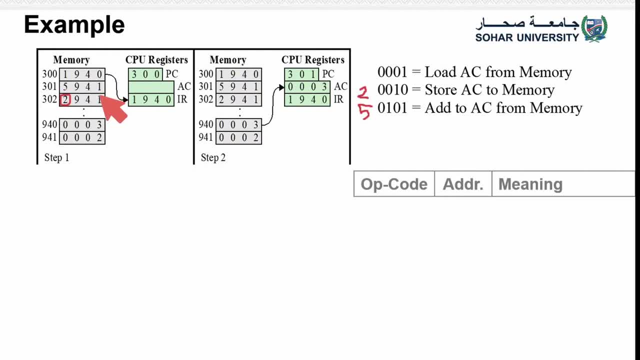 function. so bc counter the program function. so bc counter the program, counter, counter, counter. it stores the next, it stores the next, it stores the next. okay, okay, okay, the next, the next, the next address in the memory. okay so if we address in the memory. okay so if we. 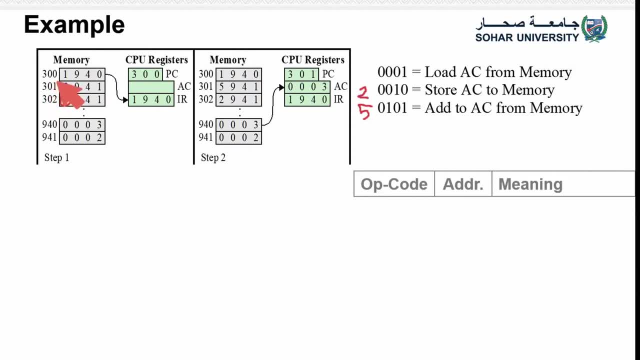 address in the memory. okay, so if we finish this address, finish this address, finish this address. this is going to be 301, this is going to be 301. this is going to be 301. when we finish 301, 301 and we execute. when we finish 301, 301 and we execute. 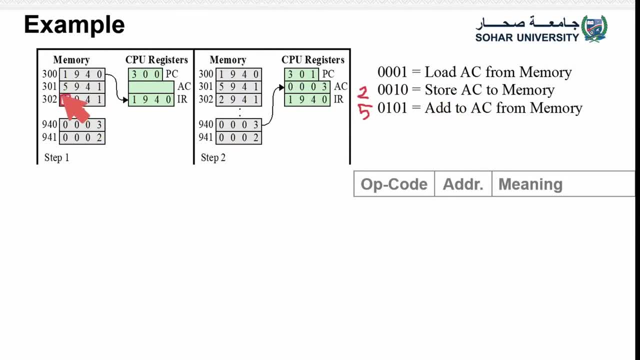 when we finish 301, 301 and we execute the uh, the uh, the uh, add instruction. okay, it's gonna go to add instruction. okay, it's gonna go to add instruction. okay, it's gonna go to 302, 302, 302, okay, okay, okay, and then it's going to execute the store. 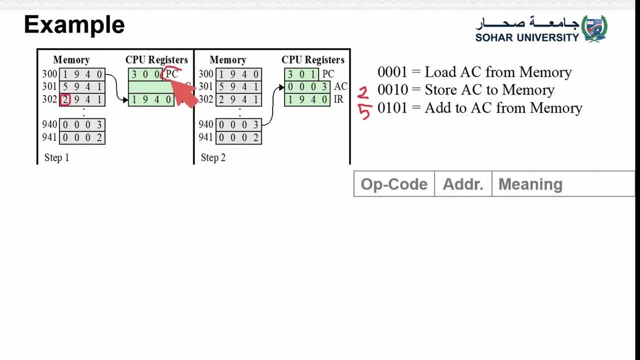 and then it's going to execute the store and then it's going to execute the store. instruction okay, instruction okay, instruction, okay. so the pc counter is so the pc counter is so. the pc counter is responsible for storing the uh, responsible for storing the uh, responsible for storing the uh, the address, in the memory. 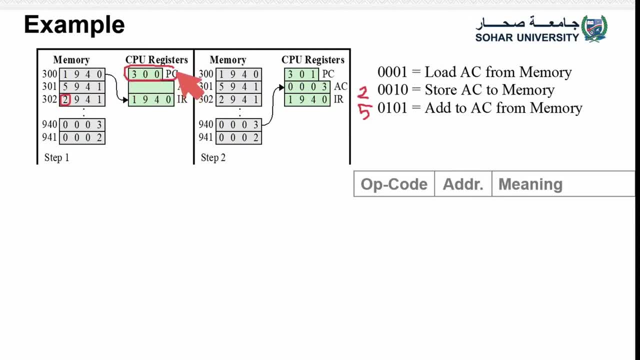 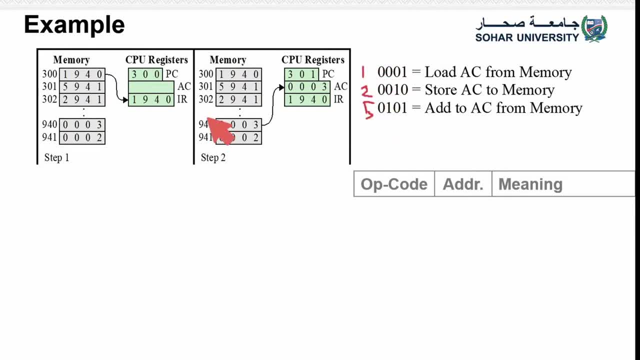 one, two and five, one, two and five, one, two and five. okay, so first we are, we are gonna look at. okay, so first we are, we are gonna look at. okay, so first we are. we are gonna look at the, the, the program counter, we are gonna look at. 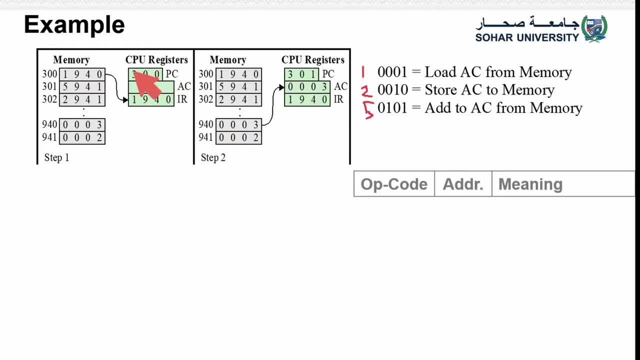 program counter. we are gonna look at program counter. we are gonna look at the program counter. the program counter is the program counter. the program counter is the program counter. the program counter is pointing at the address 300. what is pointing at the address 300? what is? 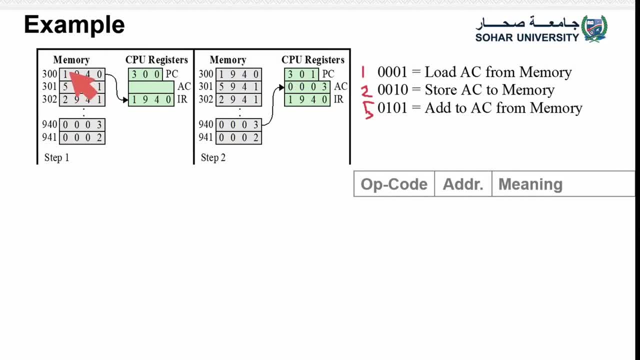 pointing at the address 300. what is inside of the address 300, inside of the address 300, inside of the address 300? first is the operation code, first is the operation code. first is the operation code. okay, so we are going to look at the. okay, so we are going to look at the. 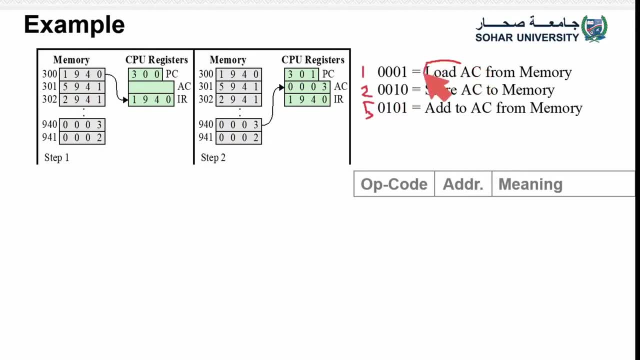 okay, so we are going to look at the operation operation operation operation code. what is the operation code load code? what is the operation code load code? what is the operation code load? we are going to load something inside of. we are going to load something inside of. we are going to load something inside of the memory. 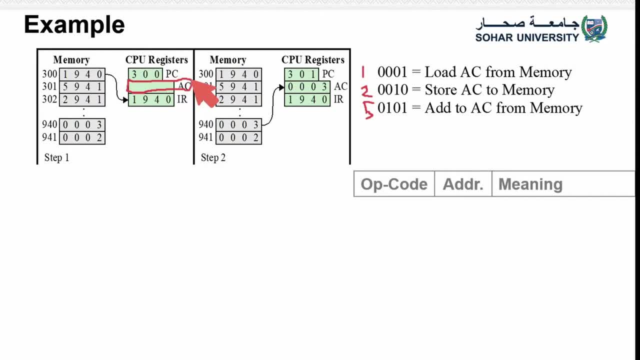 the memory, the memory into the accumulator register. so we will, we will load something from, so we will. we will load something from, so we will. we will load something from the memory into the accumulator register, the memory into the accumulator register, the memory into the accumulator register, and then we have the. 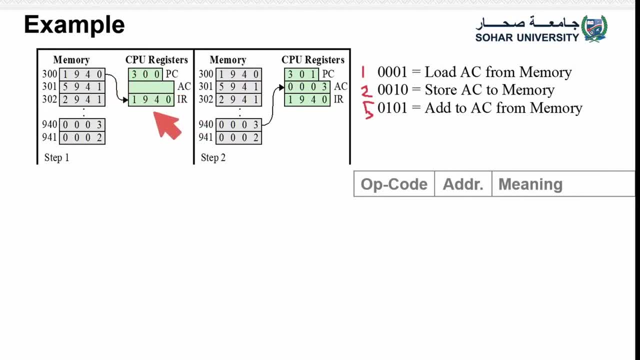 and then we have the, the instruction register. the instruction register is going to load anything that is inside of the, the address. so it's going to load the instruction, which is load, and then the address which we will load the value from. okay, so this 940 is here, this is the value or this is the. 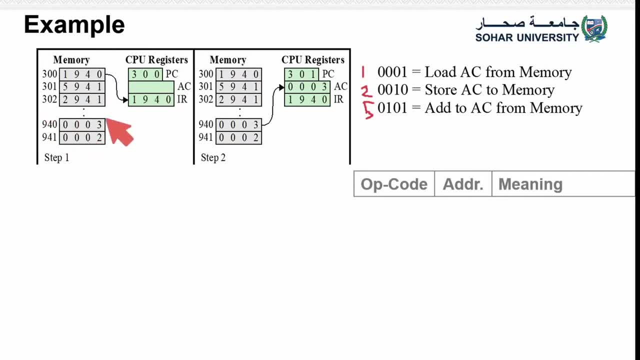 address that we want to load the value from. okay, so 940 is responsible for storing the number three. okay, so we are gonna, first we are gonna load, which is the operation code one: load 940. the address 940. anything that is inside of here, we will load it inside, inside of the accumulator register. okay, so it is here, as you can see this. 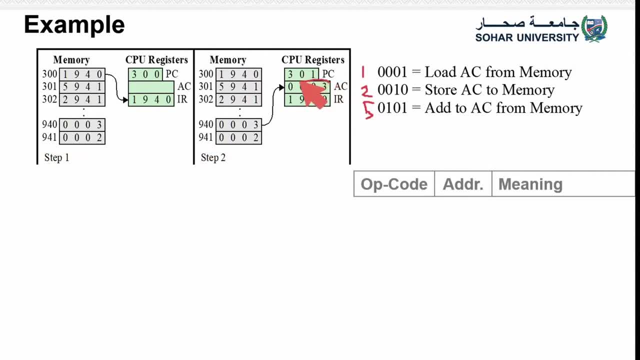 is step one, this is step two and, as you can see, here we are putting the three- okay three- inside of the accumulator register and i i told you the program counter, when it finishes the first address, it's gonna go to the address under it. okay, so here 300 and 300 only, and then here 301. so what is inside of 301? 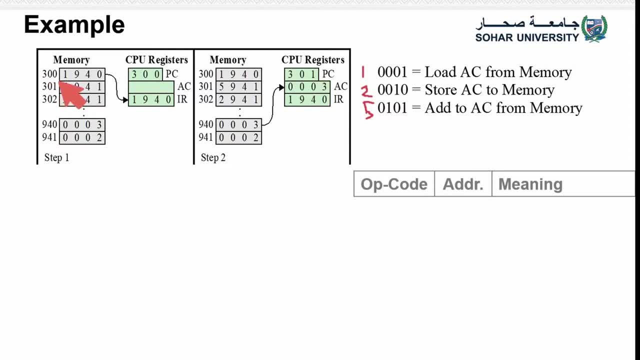 301 is responsible for the operation code five. okay, so 301 stores the operation code code 305 and the address in which we will do the calculation from. okay, so the operation code five is equal to add to accumulator from memory. okay, so we are gonna add to the accumulator, which is: 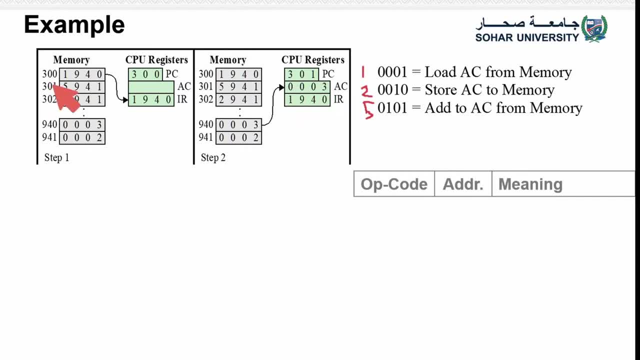 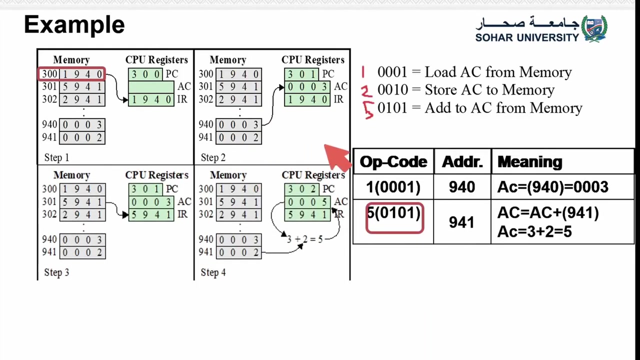 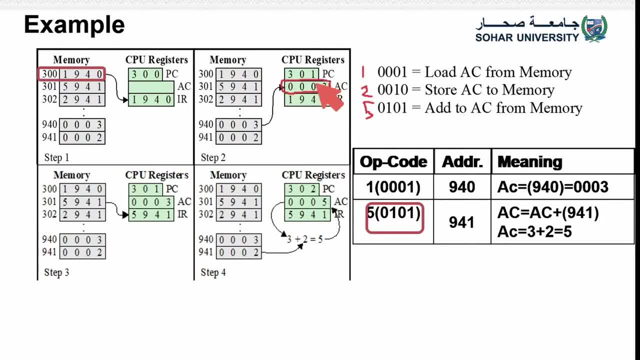 put the value three inside of the accumulator register and then the PC Counter went from 300 and 300 to 301 and then over here in step number three. okay, the instruction register. okay, instruction register is gonna load the instruction at. okay, it's gonna add what is inside of here, inside of this address, which is here: 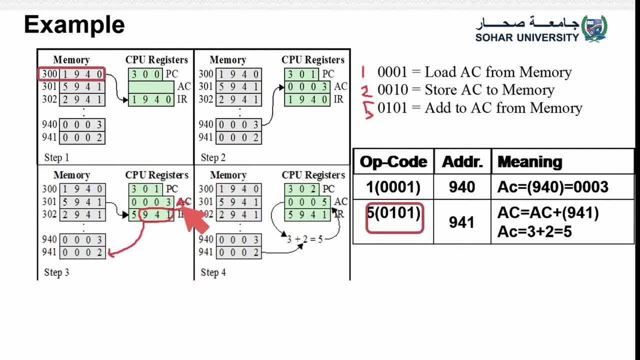 into this one. so it's going to be, as you can see here, accumulator, and then it's going to store the value inside of the accumulator, so it's going to be 3, which is inside of the accumulator. AC, AC, okay, is equal to 3, plus AC is equal to 3 plus 2, okay, as you can see here, 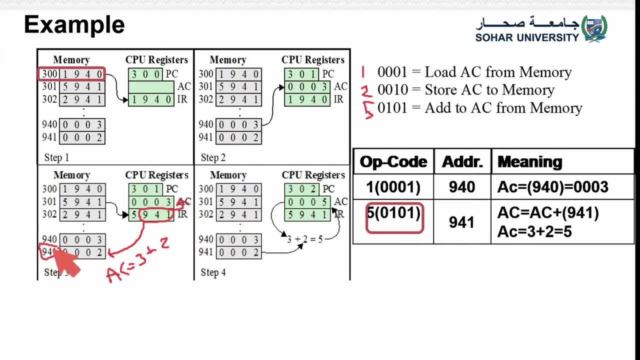 So in the address 44941,, it's going to add that value, which is 2, into this value here, 3,. okay, This is the step number 3, and then, after the step number 3,, when we finish the step number 3,. 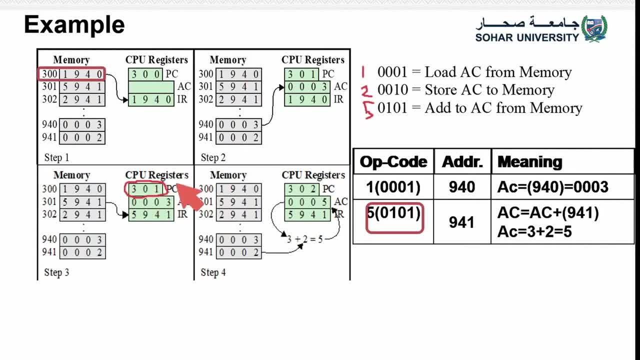 the PC counter is going to go to the next instruction, which is in the address 302,. okay, so here 302,. all right, So 302,. what does 302 have? Here is the operation code, which is 2, and, as you can see, here 2 is store. 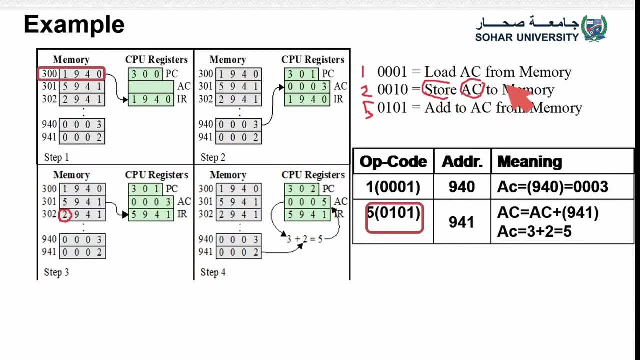 Store the value from the accumulator register to the memory. okay, So where do we store the value? here We will store the value that is inside of here, or not, that here, which is this one, 5. So 3.. 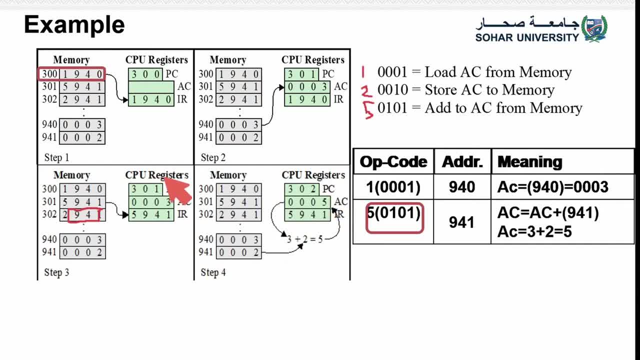 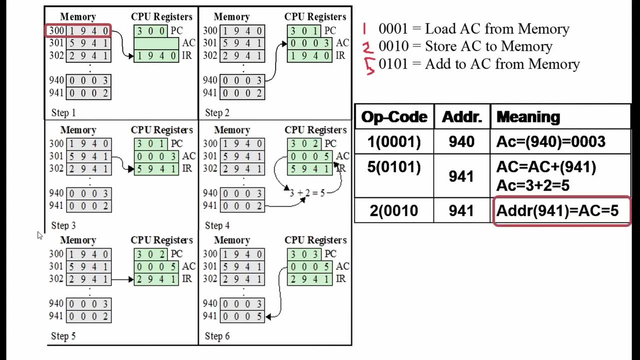 2 plus 3 is equal to 5,. okay, So this is step 4,. okay, So we are going to store the value inside of the instruction. Let me go to the other slide. Okay, so, in step 5, after we finish this instruction. okay, after we finish the instruction 301,. 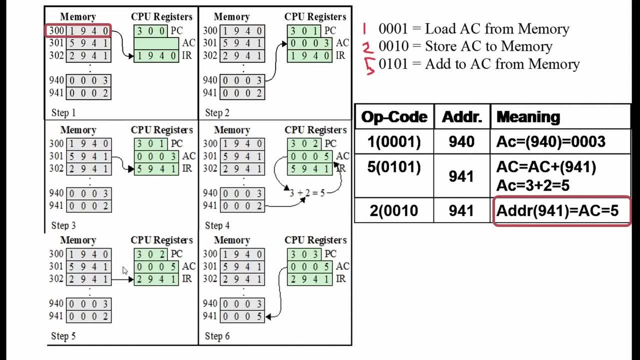 and we're going to go to the 302, which is here. The operation code is going to be 2, store, and then the address is going to be 941.. So we are going to store what is inside of here to here, okay.